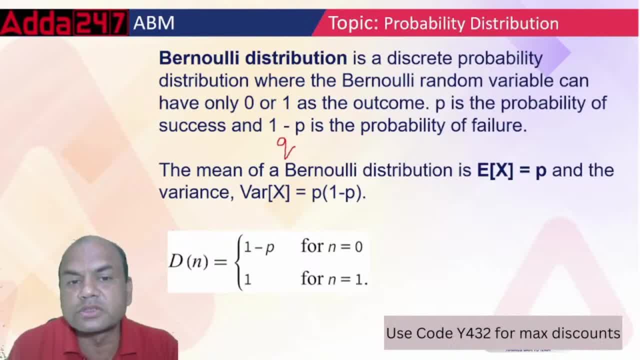 So now I see have either two answers should be applicable over here, either 0 or 1. remember important part: There should be only two answers. For example, coin suppose. if I toss a coin, throw a coin in there again, what are the possibilities? only to answer either head or tail: will you clear your CIB? only to 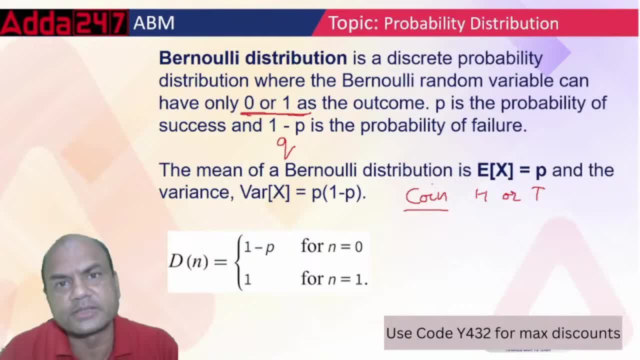 answer. either you clear it or you won't. it's that simple. so only two answer should be possible. okay, suppose if I throw a dice- dice, you know the dice we played in a school time. now it is also. we played Ludo and all those things. so 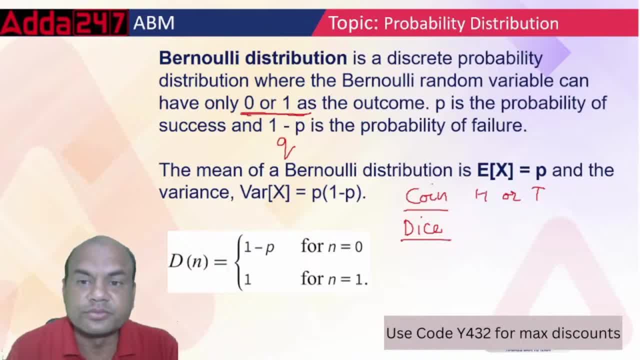 when you throw the dice, then what either you get? now there are six options: one, two, three, four, five. six means how come two? that is possible, either get six or other than six, six or other if I have to get six on the top or other, so it's. 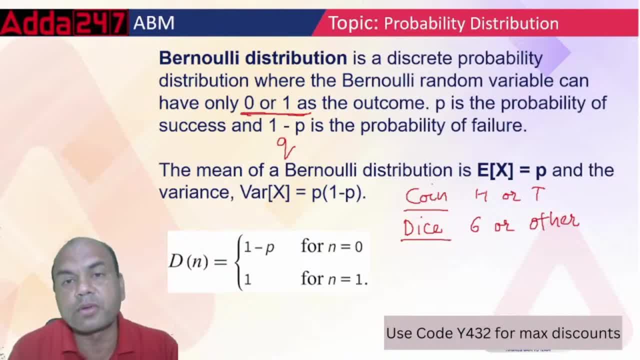 again too. so then, this way these problems are framed, so there can be only two answers, remember, zero or one, as P is a probability of success and Q is a probability of failure. now, success means, for success means that probability which is asked in the question. if they 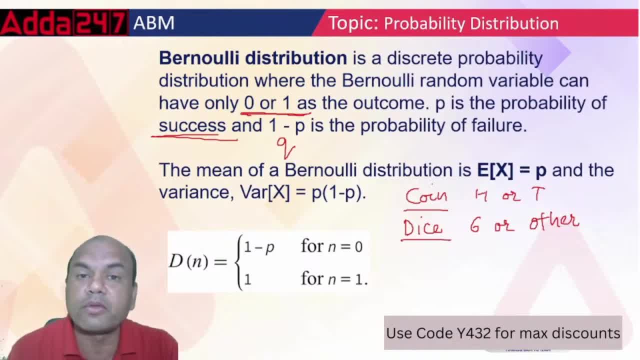 ask you, if I throw a coin and what is the probability of getting head, then that getting the head becomes a success and getting the tail becomes a failure. okay, the mean of Bernoulli distribution is: ex equals to p and variance is p into q, means p into q basically. 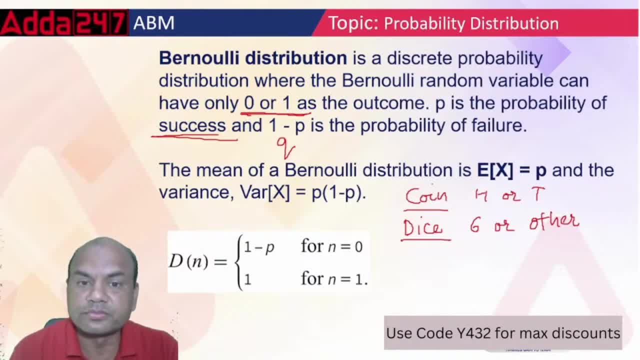 so Bernoulli is p into q. okay, variance got it simple. now this dp. so p, p equals to 1, for n equals to 1 and n equals to 0. it is q 1 minus p. okay, so remember this: either it is success or 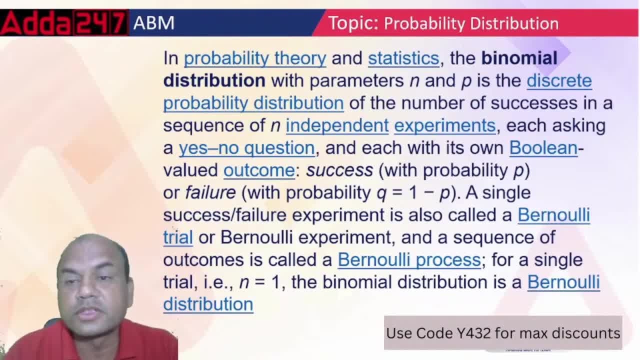 failure, simple. now let's go to this binomial distribution. now, if we, if I go on repeating Bernoulli 10 times, then that is called as binomial in probability distribution theory and statistics. binomial distribution where parameter n and p is discrete probability distribution of number of successes in the sequence of n independent experiments each. 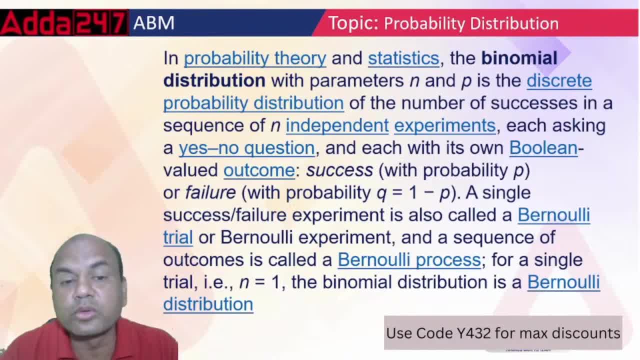 asking for yes, no questions and each with its own Boolean valued outcome. you can see that the probability distribution of n independent experiments is n independent. my god, such a big definition, isn't it? success, p and failure: q, 1 minus p. a single success or failure experiment is called as Bernoulli and a, or a Bernoulli experiment and a sequence of 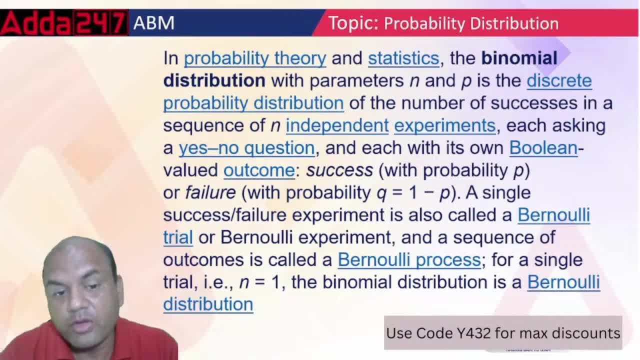 outcomes is called as Bernoulli process. for a single trial that is n equal to 1, the binomial distribution is Bernoulli distribution. I'll explain you in simple words over here. what does it mean if I go on when I do toss the coin only once? coin when I toss it only once, then it is Bernoulli, when I toss it more. 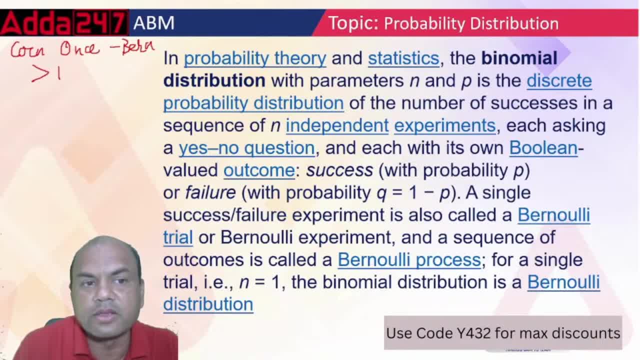 than once, more than once, greater than 1, then it becomes binary. so basically, logic is binomial. logic over here is: if I go on repeating the Bernoulli distribution, I'll get binary. I'll go on repeating it, okay, for n number of times, I'll get binary. I'll go on repeating it, okay, for n number. 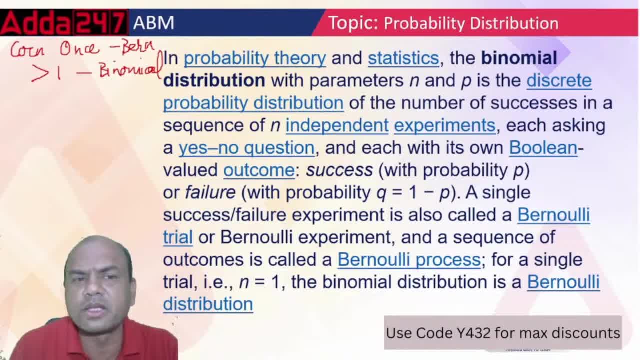 of times. so that is the basic logic. remember that much learning. each trial is independent in binomial because each trial is Bernoulli, each trial is having its own header, tail, right? so that is binomial. suppose, if I ask you in question, I'm tossing a coin five times, five times one time I'm 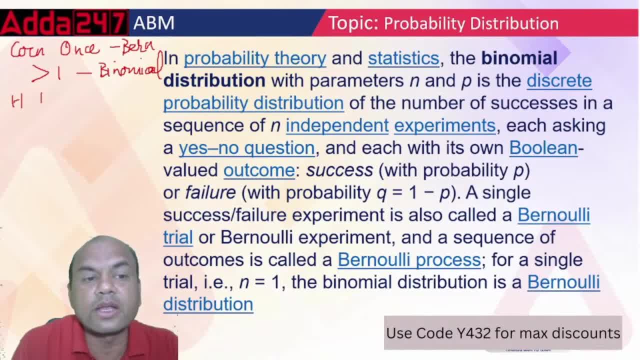 getting head. I got head over here. then again I got head. third time also I got head. so now fourth time me. everyone type in the comment section three times. i've got a head, now fourth time. can you get? guarantee me that i'll get a head again? just type head or tail, or you don't know, yes or no. 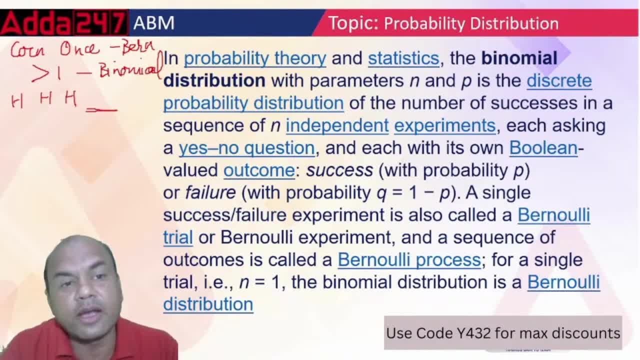 just type yes or no. can you guarantee me that you'll get a head again over here? you can't guarantee me why? because each trial is independent. suppose, if i get two times and i can't guarantee that third time i'll get ahead, fourth time i'll get ahead. fifth time i'll get it. so that's why. 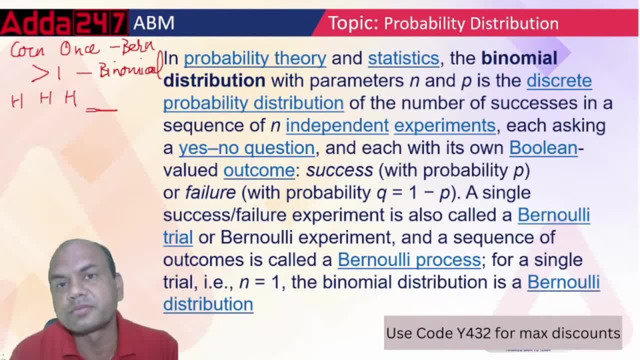 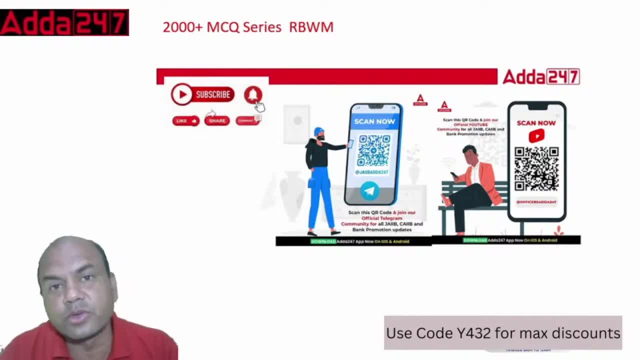 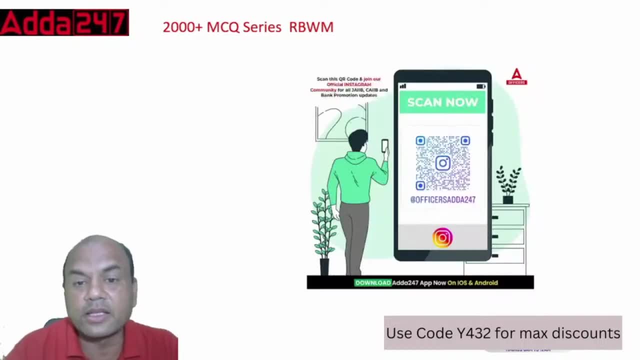 binomial means each time it's a bernoulli experiment and each trial is independent. okay, now, before going ahead, everyone scan these qr codes. this blue one is for our linkedin channel, this black one is for our youtube channel and this other one green one, or this blue, this? 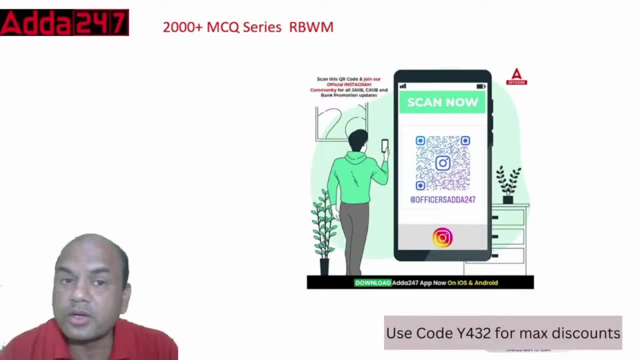 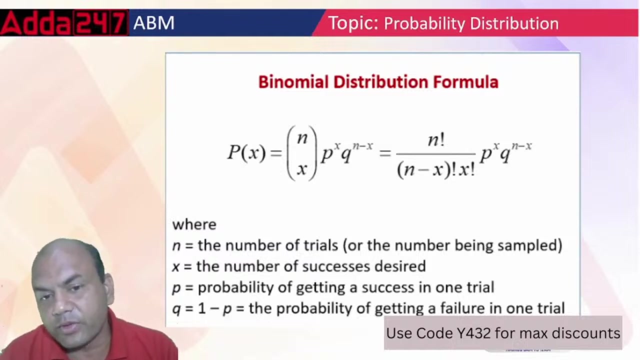 this is for our instagram channel. if you join all these channels, linkedin instagram as well as youtube, because we provided various free youtube series. number one, secondly, we provide with free questions, question banks, free tests on this channel, so that's why join immediately. okay, now binomial. this is a formula for binomial: ncr into p raise. 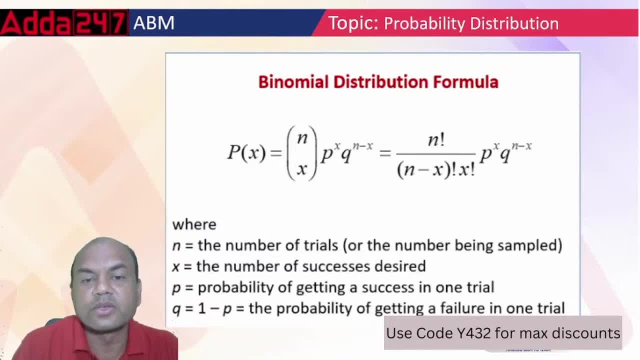 to r. q raise to n minus r or x. we call it so ncx. p raise to x, q raise to n minus x. n is number of success is required. number success is required, okay, p is the probability of getting success in each trial, single trial, and q is the failure: probability of getting the failure. so this is: 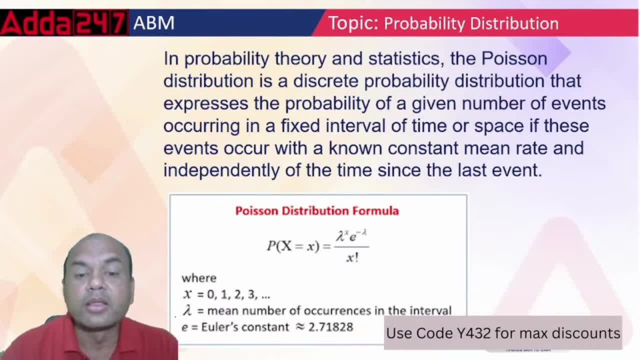 binomial. now if you go on in poison, in probability distribution theory and statistics, the poison distribution is a discrete probability probability distribution that expresses the probability of probability of success given number of events occurring in fixed intervals of time or space, if these events occur with a constant mean rate. now one thing i'll clarify over here: poison distribution, remember. 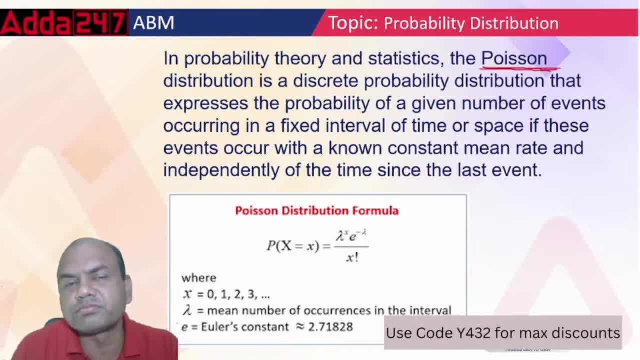 in exam you will always face the problem like how to identify. this problem is a bernoulli binomial or poison, how to identify? so to identify that, remember in binomial you will always get. each trial should be independent, very important. each trial means you shouldn't be able to guarantee the next trial. 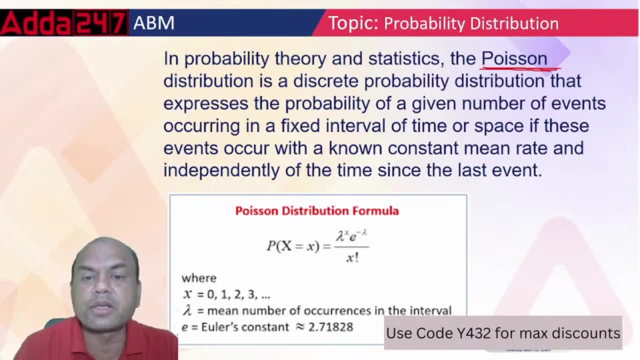 whether i will get head or tail and for poison. always remember there will be something constant over here, fixed interval, something constant, okay, something fixed, something constant like the like. suppose example: you are getting some virus every two hours. you are getting, you are getting almost two, three deaths. 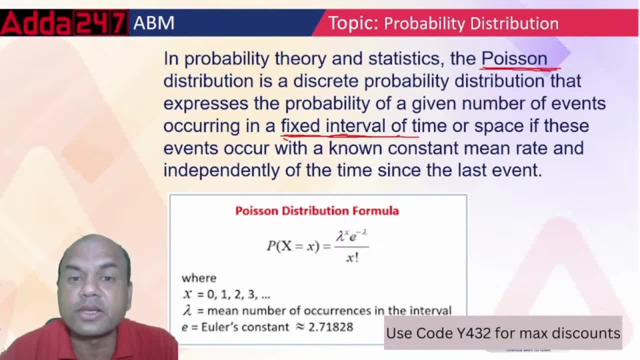 or three patients, why? that's okay, three patients every two hours i am getting, so this is a constant phenomena. so poison will always see this constant phenomena. for example, electricity in a city or in an area. every day, three hours, electricity is not there, so this is a constant phenomena. 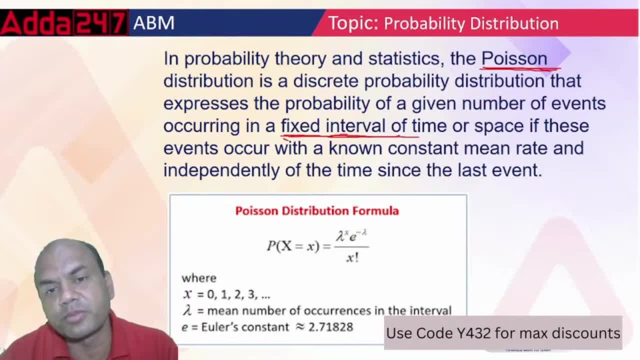 from when you get such problems, you understand that it's a poison problem. what is the formula for poison series? the formula for poison is this: lambda raised to lambda, raised to x, you can call it or e. raised to minus. lambda upon x, factorial. okay, what is x required? x equals to 0, 1, 2, 3, whatever is required. 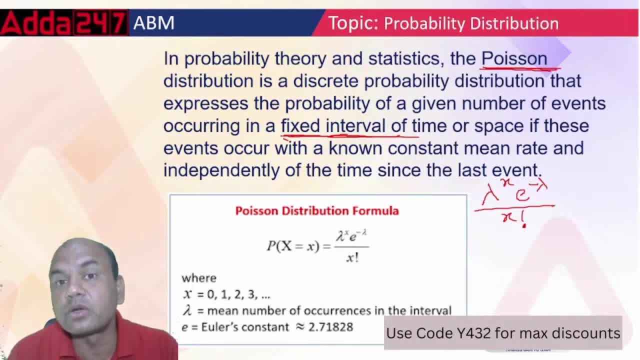 lambda is a constant thing happening, which is happening constantly. two hours, every two hours electricity is gone. per day, two hours electricity is not there. so that is the constant thing and e is known as euler's constant. it is 2.72, roughly 2.718. it's a big number, but you can consider it 2.72 simple. okay. so this is poison. 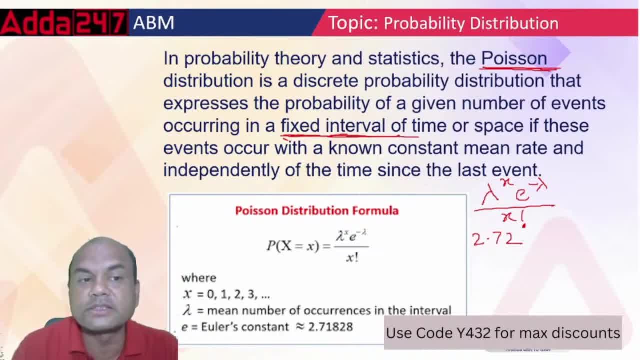 so binomial formula. what is the formula for binomial? ncr, ncr, p raised to r. q raised to n minus r? right, what is the formula for this poison? lambda raised to x or r, you can call it here, some books call it r, some books call it s one and the same thing: lambda raised to r. e raised to minus lambda. 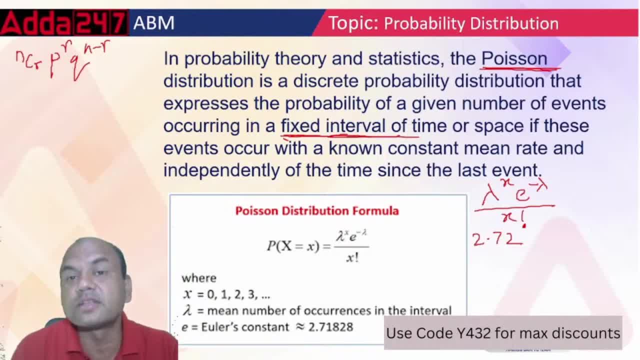 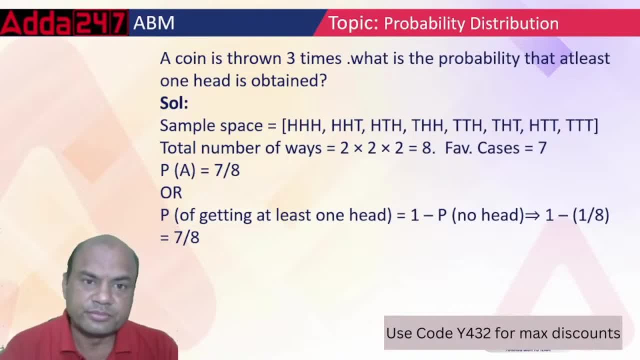 upon r factor. okay, what is r or x? it is what is asked in the exam. okay, so that was the theory part. now we'll solve some numericals. okay, so theory, everyone got it type yes in the comment section. you must, from this lecture, you must at least understand the formula and for binomial and 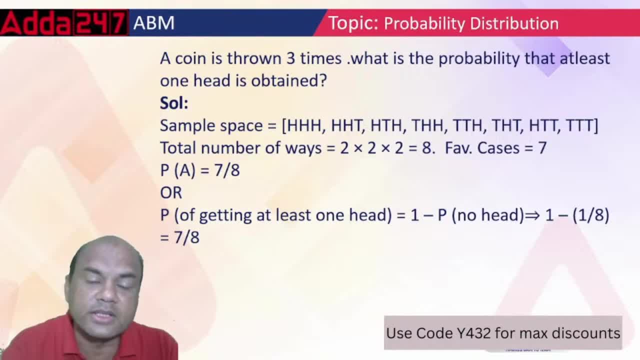 this poison okay. so have you got this now? shall we move ahead? now type yes in the comment section. everyone yes. type yes, okay, move on. a coin is thrown three times. what is the probability that at least one head is obtained? see, a coin is thrown three times. three times, i am throwing a throwing. 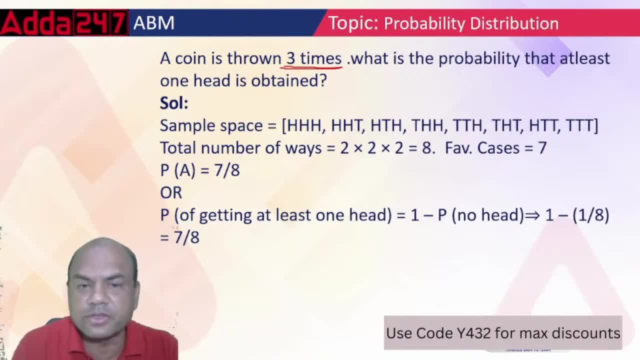 the coin. so three times means what? suppose if i throw the coin only once here? once i throw the coin, what is the possible possibility of getting? the answer means either i'll get what- head or tail, Right, Simple: If I throw the coin only once, I will get head or tail. So what are the total outcomes? Two, If I throw the coin two times, two times. so again I might get head or tail, or tail or head, anything, isn't it? 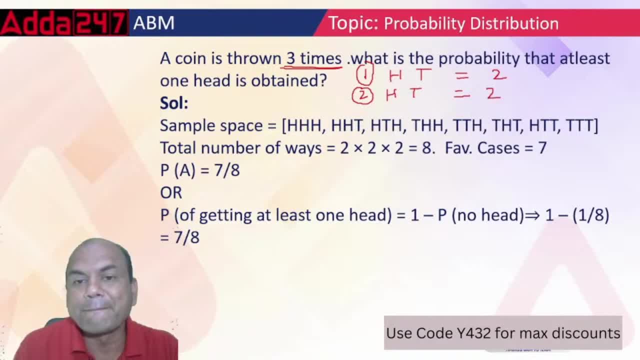 So again, what are the outcomes? Two, Right Now. third time: three times I am throwing. Third time. So now look at this: The outcomes over here are two. So two times I am throwing it, But the answer doesn't. third time, the answer is not six. 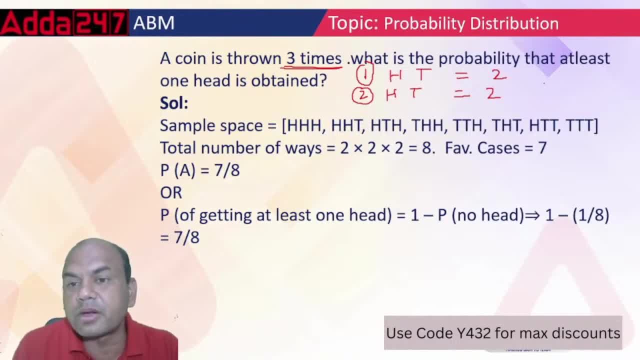 So if I throw the coin three times, the outcome is, remember, two raised to zero. Two is the outcome for each raised to three. So the outcome will be eight possibilities. Now look at this. Look at these possibilities. See this: Eight possibilities, because I am joining them three times. Three times I am throwing the coin, So there are eight possibilities available. Suppose, if I throw the coin four times, then it is two raised to four, Sixteen. Okay, So now find the answer. It is either HHH, See here, three times I am throwing the coin So I can get all the heads also, or head, head tail, or head tail, head, tail, head. 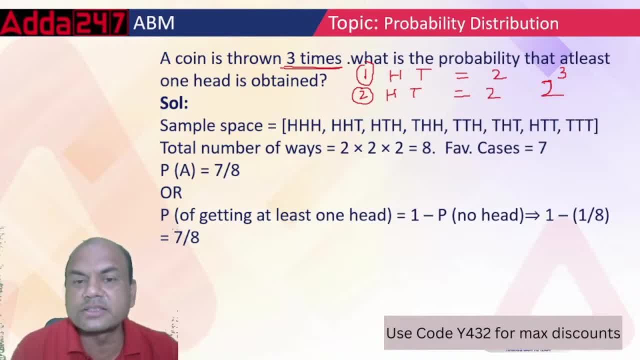 All this Here. you see this. These are eight possibilities. Now, what is asked in the question? What is the probability that at least one head is obtained? At least one head. So now am I having one head over here? Yeah, I'm having more than one head. So this is okay. This is okay. 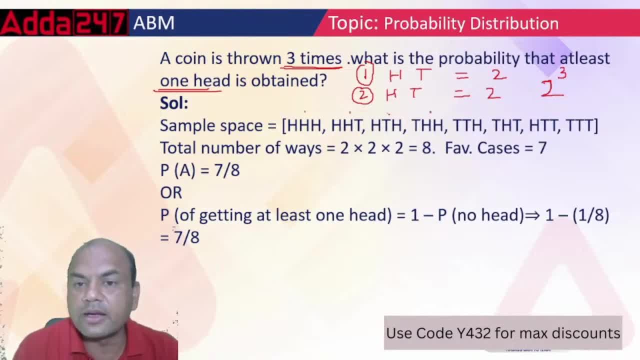 Head head, tail head- Okay. Tail head head- Okay, Tail, tail head- Okay. One head, at least one head. I am scared. This also. This is not okay, because here i am getting tail, tail, tail, so this is not okay. so how many are the required successes? 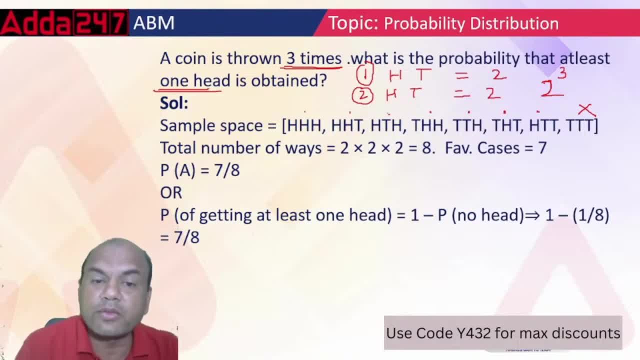 over here. see at least one head. so what is the formula for probability? probability is always the success, probability equals to success or p success. basically, upon sample space: total number of elements. total number of sample points means whatever are the sample points available or what is order the sample space. so what is the sample space over here? sample space means total number. 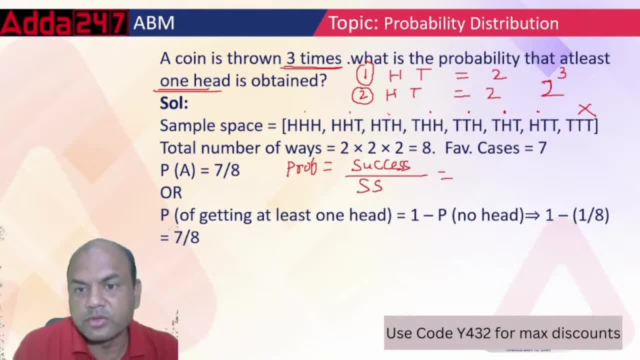 of outcomes. so how many outcomes are there? eight. so here i am getting eight outcomes. how many successes are required here? at least one head. so it is seven successes. so my probability becomes seven. seven upon it. so that is my answer. seven upon it. right now, suppose, if i ask you find the 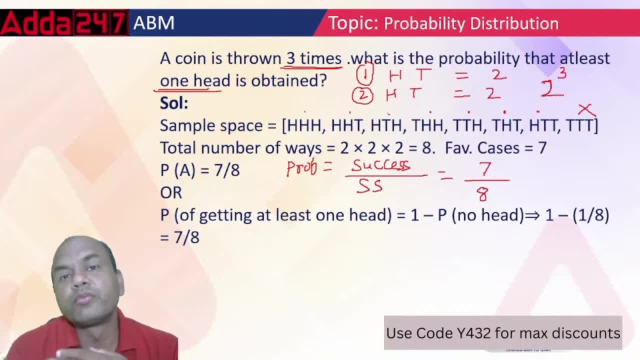 probability. everyone type in the comment section: now everyone got this problem by now, got it everyone. now if i ask you what is the probability that you will get no head? no, i don't want any head now. so at least one head was seven upon it, so no head. 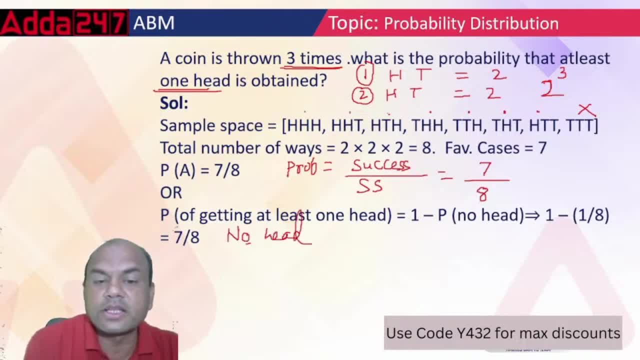 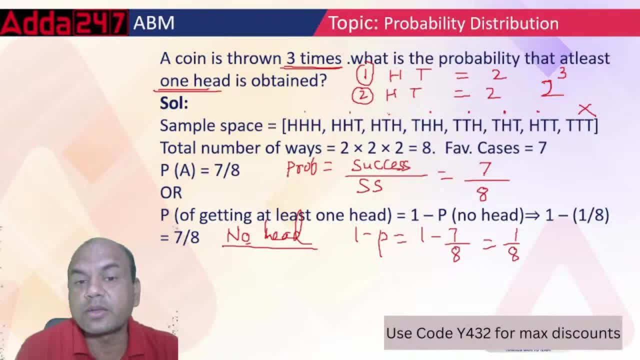 least two heads. two heads. so in that case, what can be the possibility- at least i am talking at least so. one, two, three, four, these four are the answers. at least two heads, right? one, two, three, four. so if i ask you two heads, then what will be the possibility? 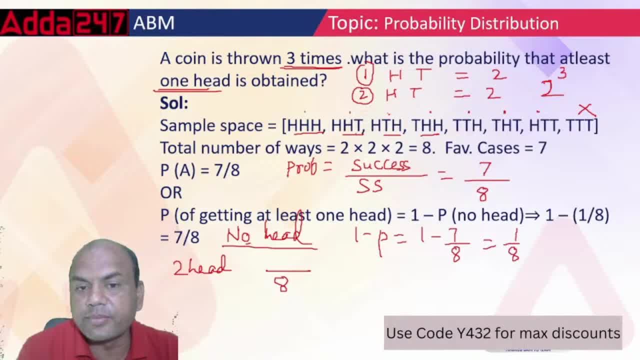 two heads, so it is: denominator is eight, but here it is four, so it is one by two. this is the way we must solve these numericals. okay, at least two heads. if i ask you, you should get at least three heads. at least three heads, then what will be the answer? 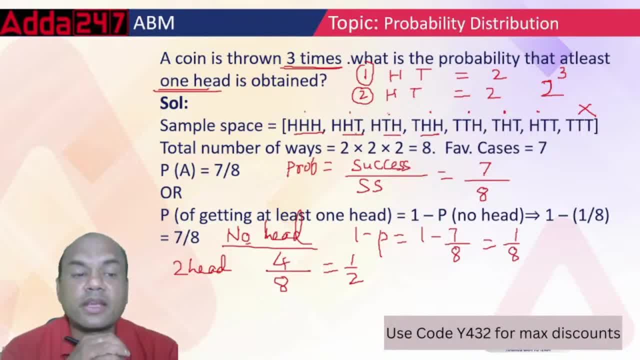 now you type in the comment section: at least three heads. i want to answer for at least three heads, everyone. yes, at least three heads deal. this does not mean that at least three heads that is the case. is it obvious or not? tell us your answer. you just take that at least three heads. 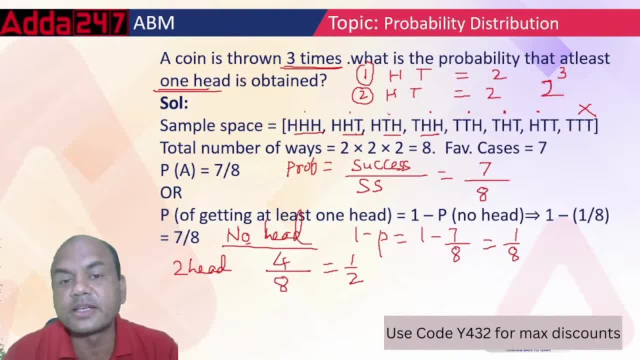 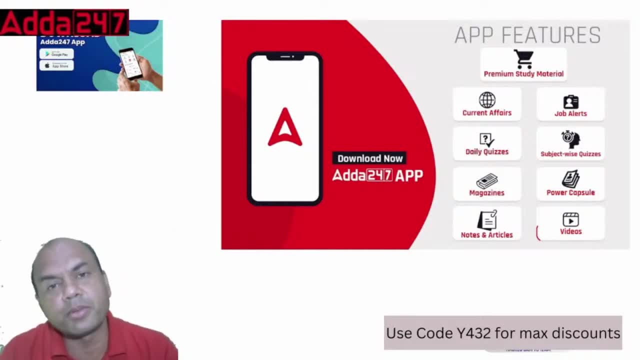 yes, at least three heads. right, what is the answer? at least three, yeah, so there's only one one up on it because everyone else is having a two heads. at least three upwards. only one, right? everyone download dot 24 7 app on your mobile. in this app, you will be getting the premium study material plus live classes, ebooks, tests. 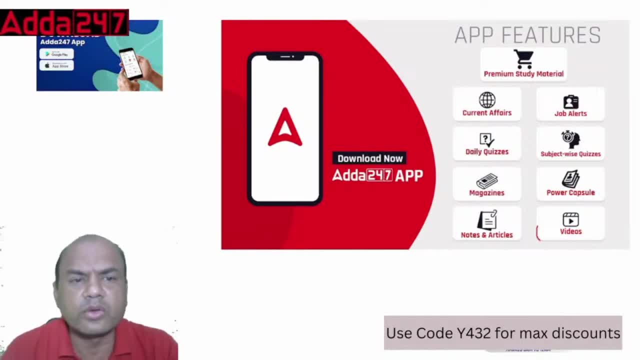 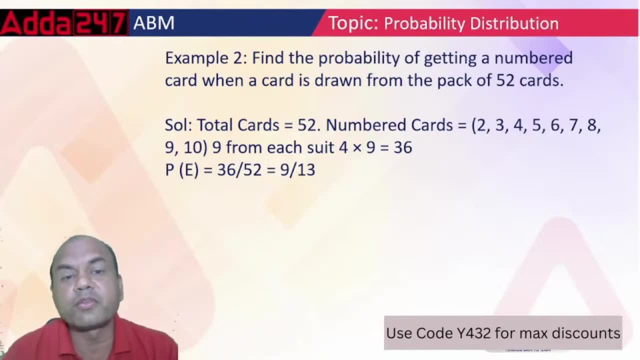 books test. you get it over here, so download it right now. download this app, share it with your friends. okay, find a probability of getting a numbered card when the card is drawn from a pack of 52 cards. now, I want a numbered card. okay, numbered card. now. how many numbered cards are there? firstly, tell me and. 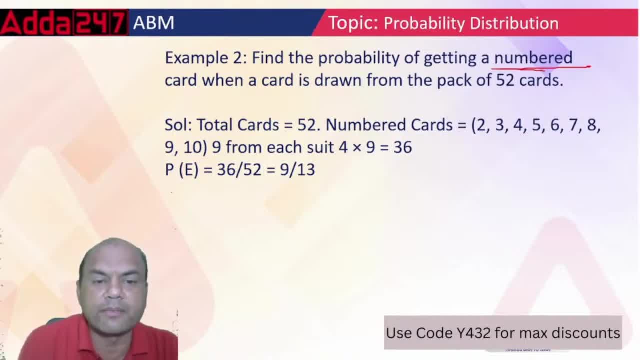 total is 52. okay, first remember the probability formula, for probability is what success? okay, upon total right sample space. so totally simple: totally awarded 52 right. total is 52 cards. what about the success? success is what numbered card? now, how many numbered cards are there in a pack of 52 cards? 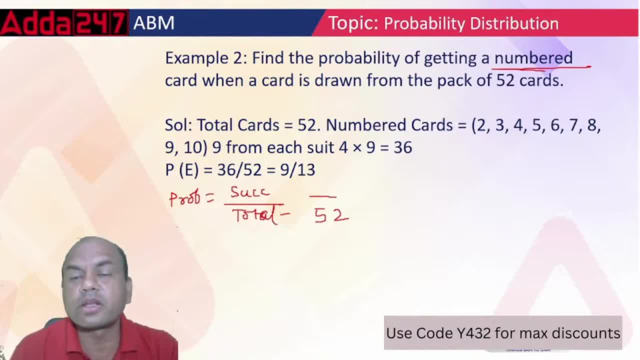 how many numbered cards here. numbered cards are what are numbered cards which are having numbers. so 2, 3, 4, 6, 7, 8, 9, 10 up to 10, you're having all the numbered cards after 10. what do you have? you have that. 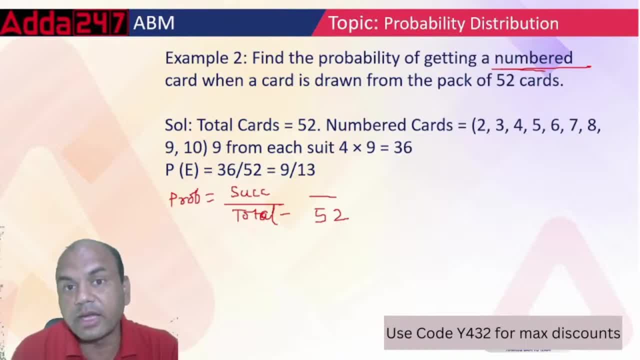 Jack, you have the Queen, you have the King and you have. that is so these are all called as what's here. remember, there are three types of facts. one is numbered, numbered okay. second one is: hmm, what is this? anyone knows? second one: yes, face card is there, but this is not answer. honor. honor card is answer. honor card. 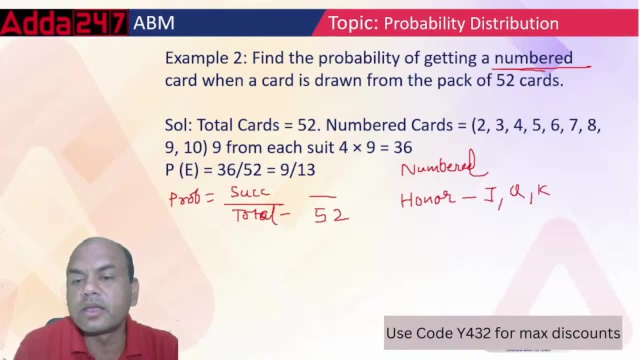 Jack, Queen, King and Ace. and last one is face card. face cards are three, only Jack, Queen and King. no, Ace is there is. does Ace have a face card? Ace means that Eka, we call it right. does it have a face? no, so here, what do I want numbered? 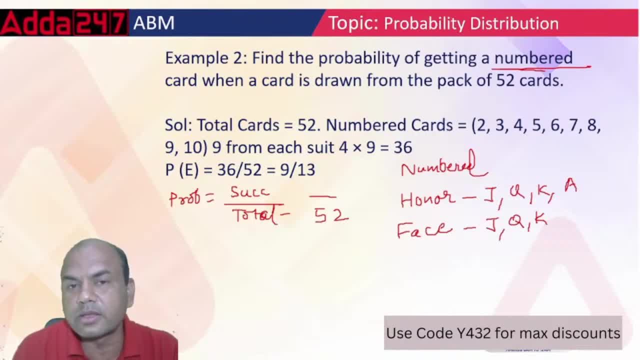 numbered means how many are there? 9, 2 to 3, 2 to 10, so there are 9, but 9 in 1. so similarly, yes, four types of cards, right, so 9, so the 36. so i'm certain will give 36 upon 52. 36 upon 52 said you go on dividing it. it was 4, 4, 9, 4, 13, 4. this is. 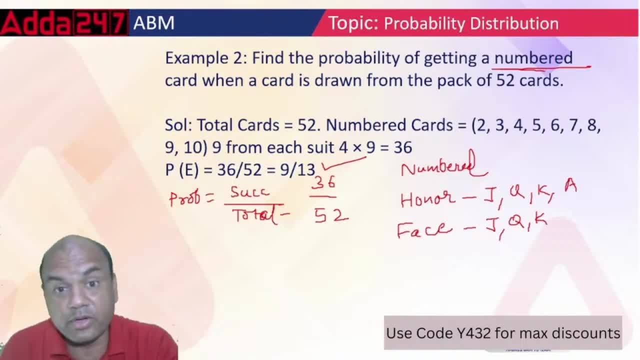 your answer. 9, method 2: everyone got this year. this is very important concept to understand. okay, you guys should understand this very properly. got it everyone clear. These were the numericals which I had told you See, here we want to do theory and numericals. 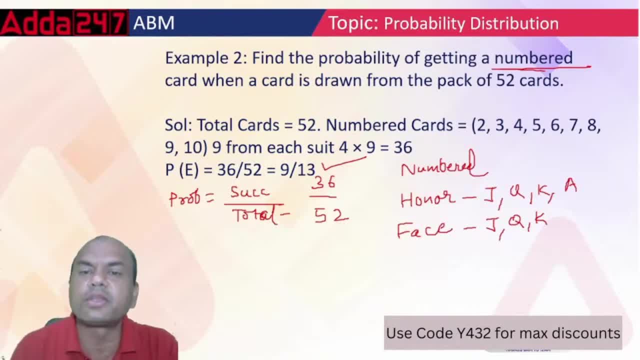 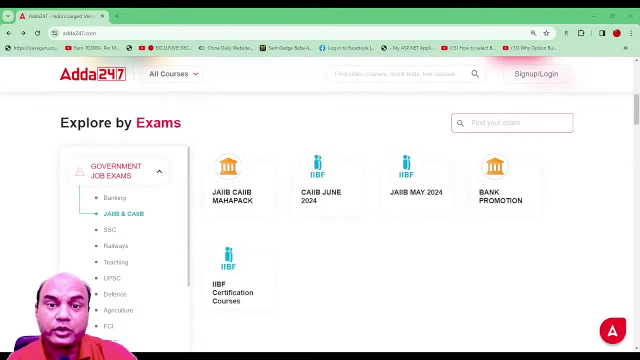 See here all the numericals. are not possible to be done in this half an hour class. Okay, That was the YT series for you. Now, before going, let me tell you join the batches immediately. See here all the numericals. objective questions, case studies- everything is covered in the batches. 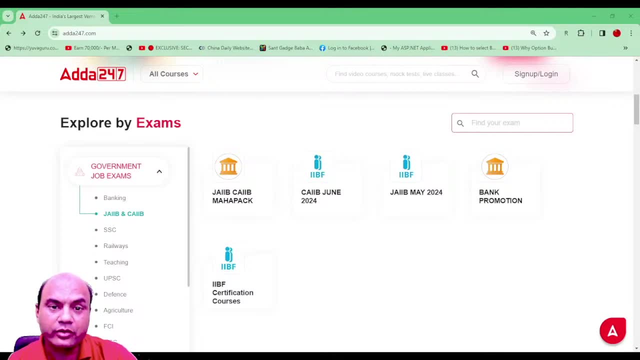 You can join the MAPEC also. Let me show you. Go to ADAT 24-7.. I will always suggest you to go through the app. In the app, you get 1% extra using the coin systems. Okay Here, go to ADAT 24-7.. 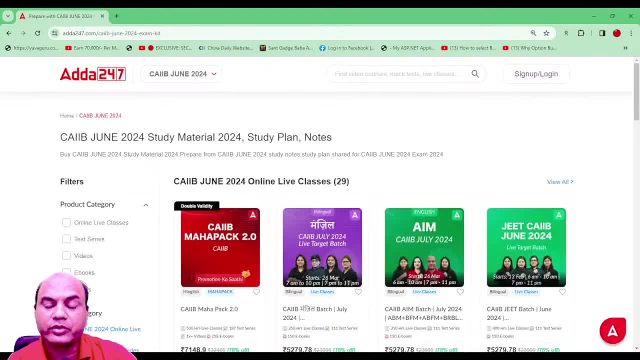 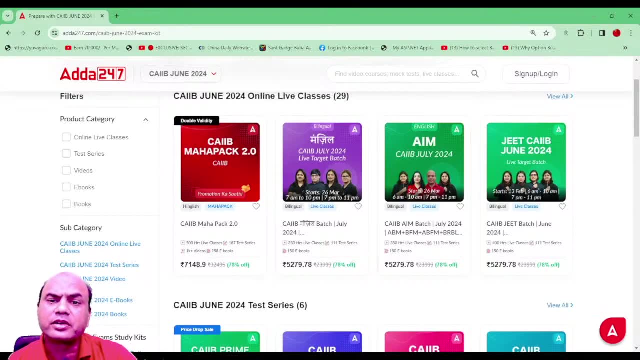 Click on JIB and CIB. Click on CIB- June 24.. Here you will see the batches. Look at this AIM batch Then you can join the batch. AIM AIM batch- It covers all the numericals. objective questions, case studies. 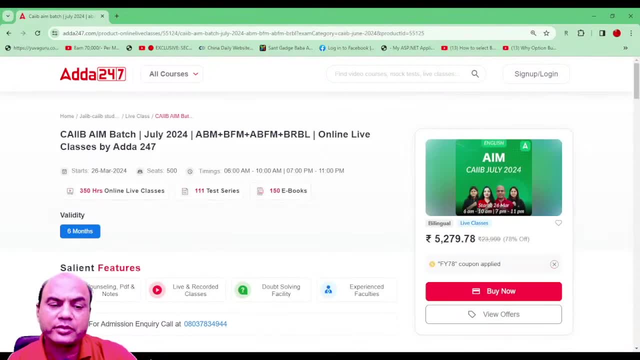 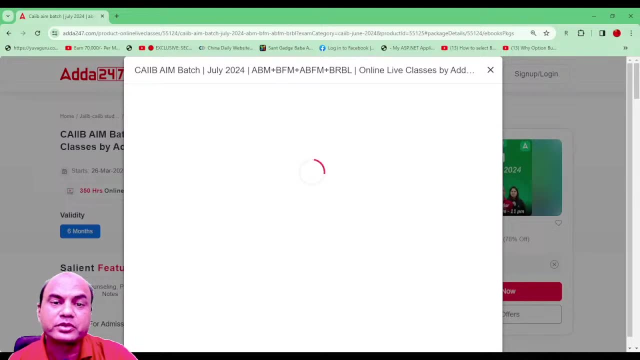 Click on this. Look at this: E-books, test series, online live classes, counseling, live recorded session- Everything is available. Click on the E-book. You get subject-wise E-books over here Now. if you click on each subject, you get module-wise, chapter-wise. 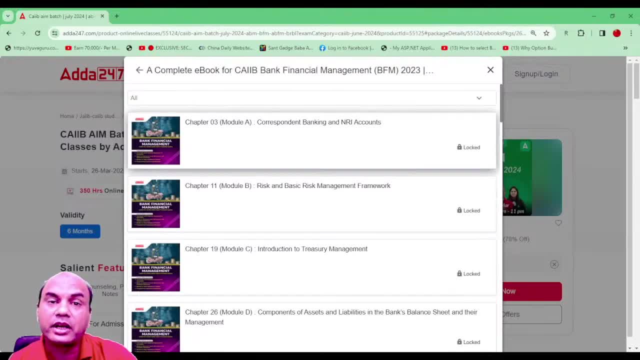 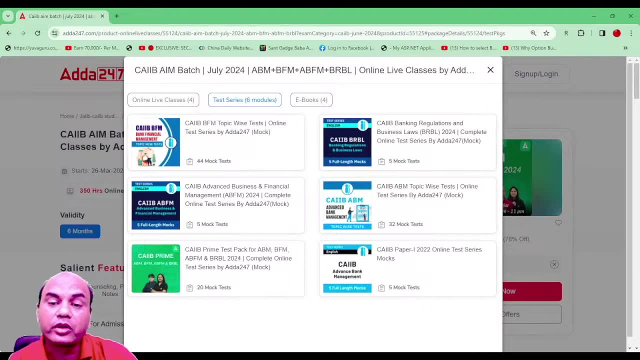 See this chapter-wise: Chapter 3, chapter 11, chapter 19.. So you are getting chapter-wise Similarly test also If you go for the test. the tests are also available module-wise and chapter-wise. Look at this.